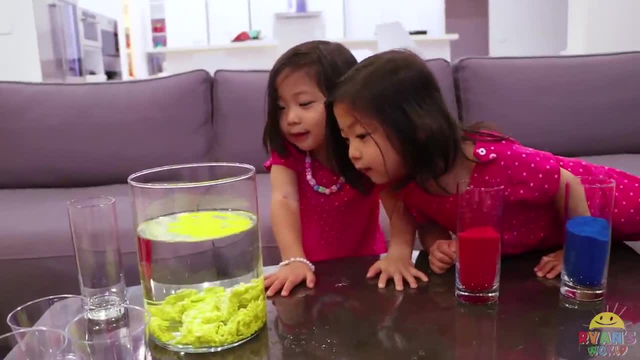 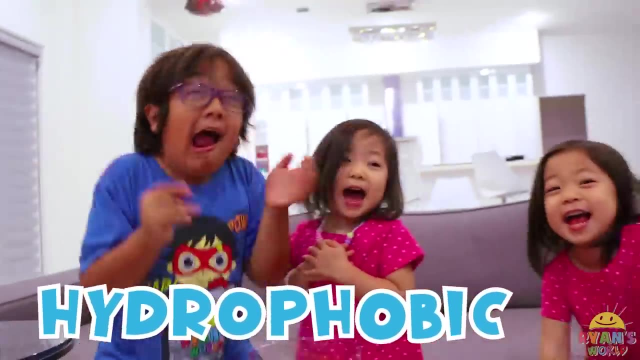 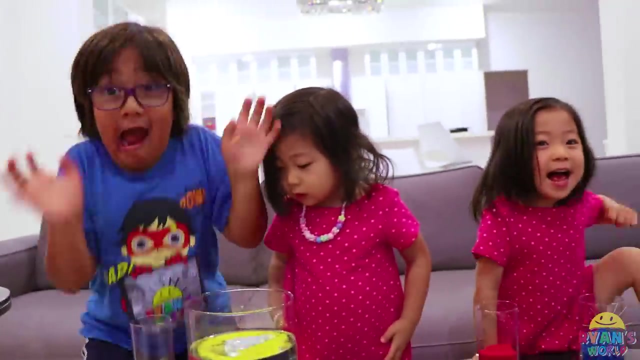 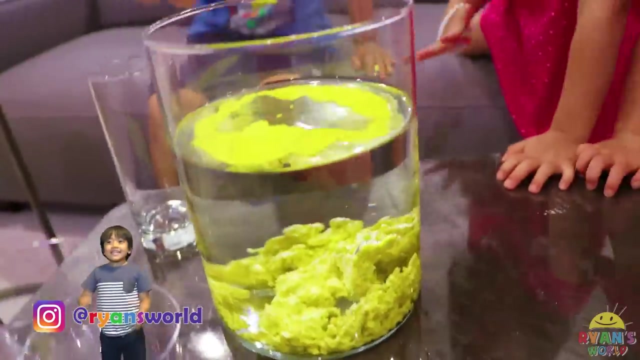 Yeah, You know what's so special about the sands? What They are hydro-phobic. Ahhh, You know what that means? No, They're scared of water, Ahhh. So they don't like to touch water. So you see how, in the sand here- look if I pick it up, instead of being wet, they become dry again. 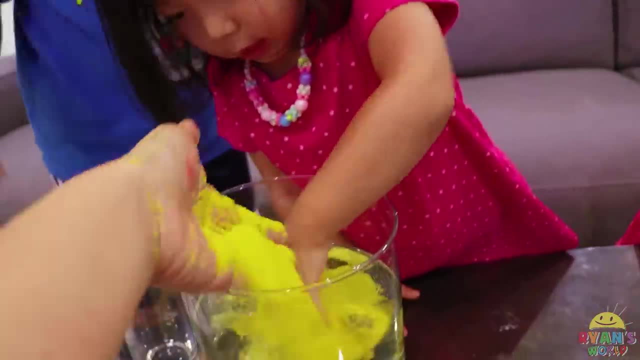 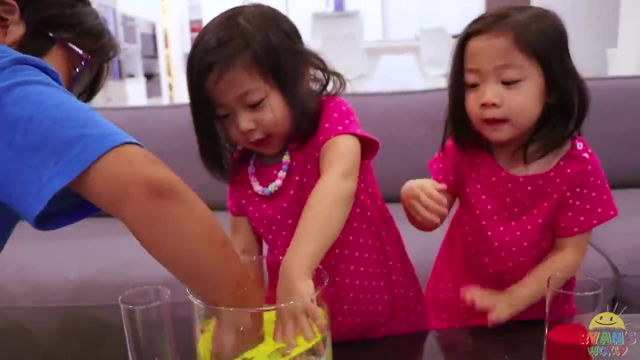 Whoa, They're dry sand. Now they're wet sand. Try it. Put your hand in there and pick it up. You think they're wet, but they're actually. pick it up and they're dry. Whoa, You see. 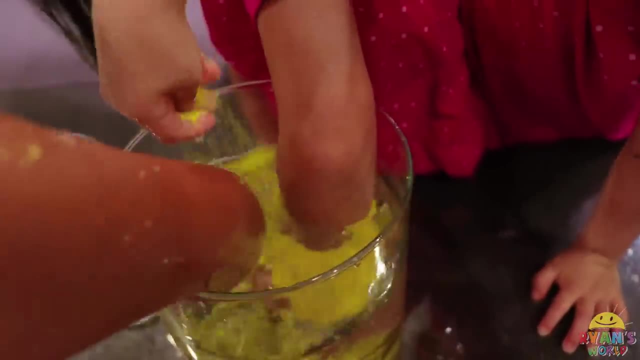 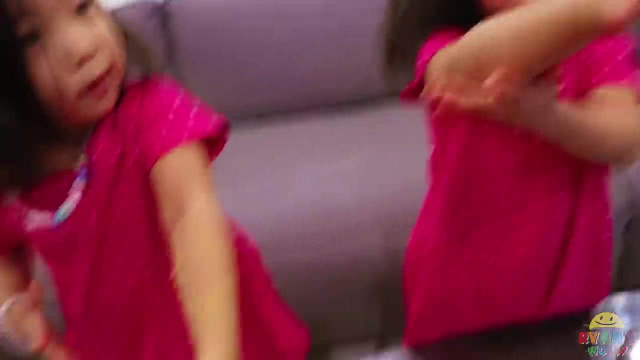 Yeah, so there is a repellent in there, A repellent in there that makes them not wet. Did you pick the sand up? What happened, Ryan? I did? Whoa, Yeah, I didn't pick it up. See, they're dry. 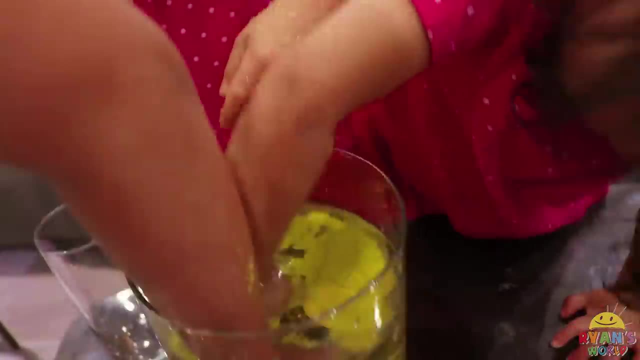 How Am I right? Isn't that cool? Yeah, Yeah, They're one with the everything. Yay, My turn, my turn. Alright, you want to try a different color? What color are you going to pick, Kate? 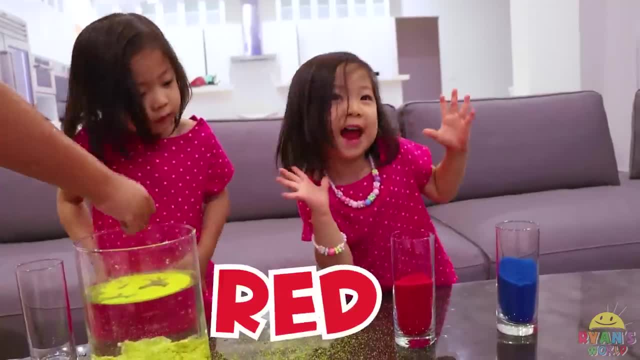 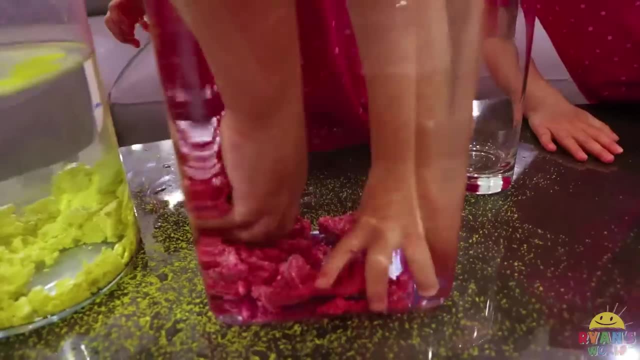 I want red, Red, Okay, Blue Kate's doing red. Do we all do different stuff? Whoa, No, they're the same. but look, Wet sand, Emma, you're going to look. Okay, I'm going to look at the sand. 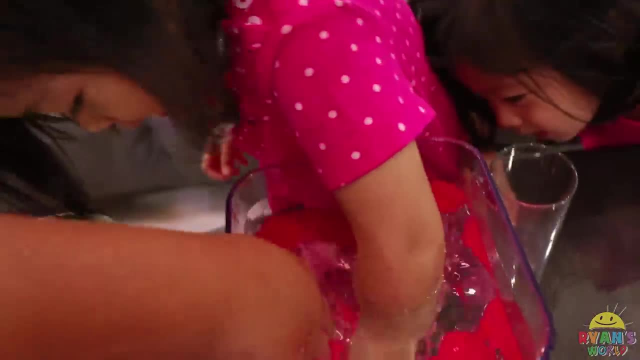 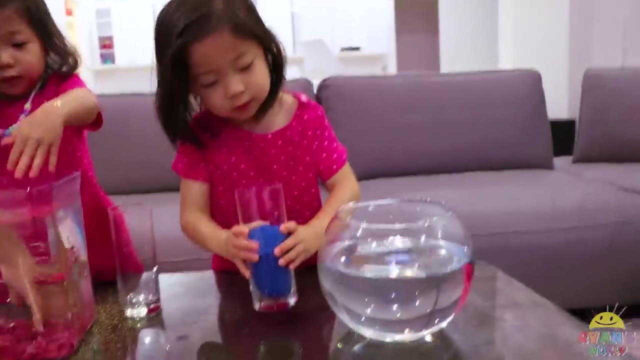 Emma, are you going to look at it? No, I'm going to dry sand. Woohoo, That was my turn. Yeah, Okay, so Emma's going to do the blue sand, and I got a fishbowl just for you, Emma. 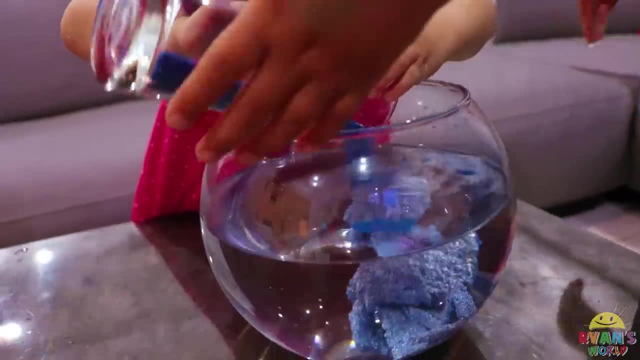 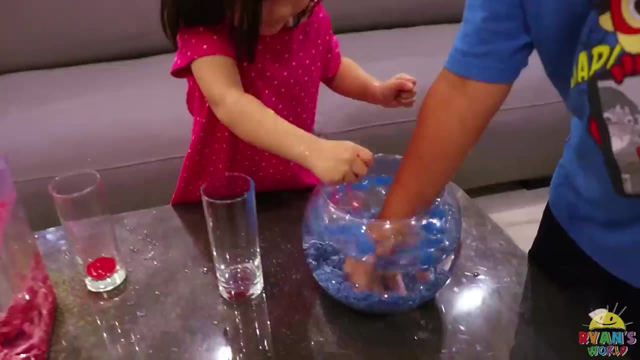 There you go Slowly. Yeah, I like it. Good job, Emma. Do it slowly. I'm going to do it. There you go. Look at that, I'm going to mix it. You're going to mix it. 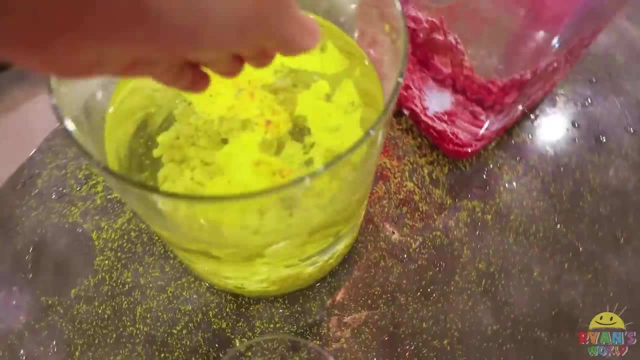 Yeah, Ryan, Oh, So you can unmix it by just picking up the sand, Look and it's all dry And you just put it back. All right, I'm going to unmix it for them because I can do it again. 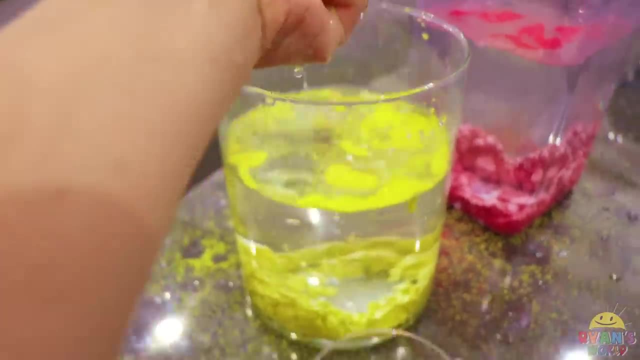 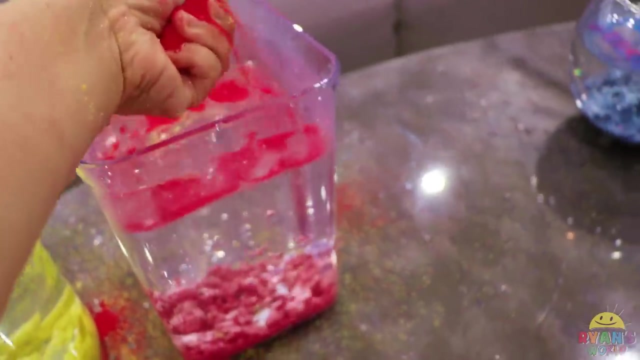 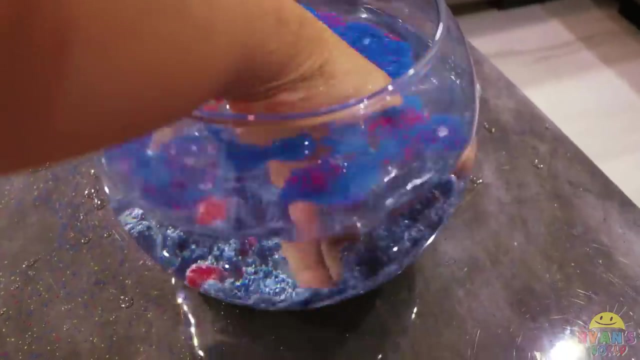 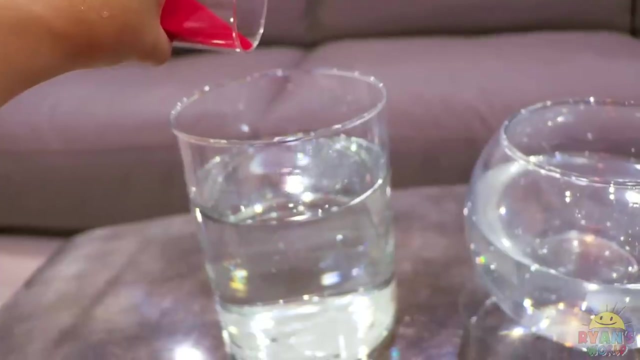 Wee. So now the red. They're up there playing. That's why the noise. Okay, Wee, I'm going to do it slow for you guys to see. Oh, Here's the blue one, slow. And now I'm going to do the yellow. 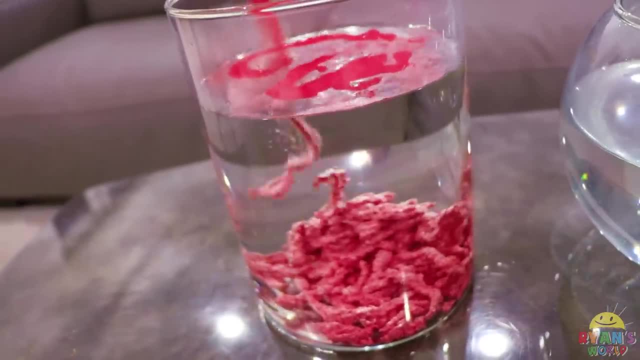 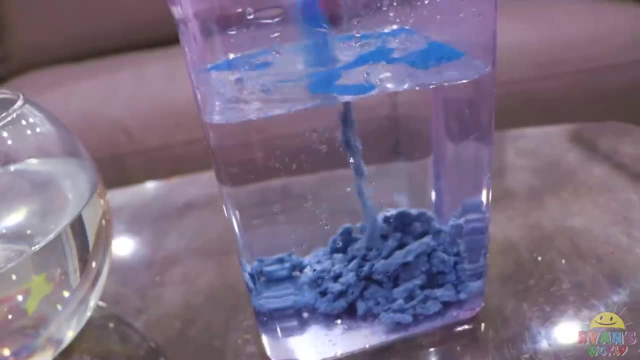 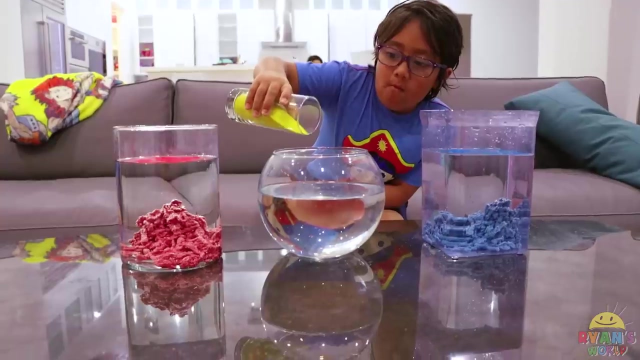 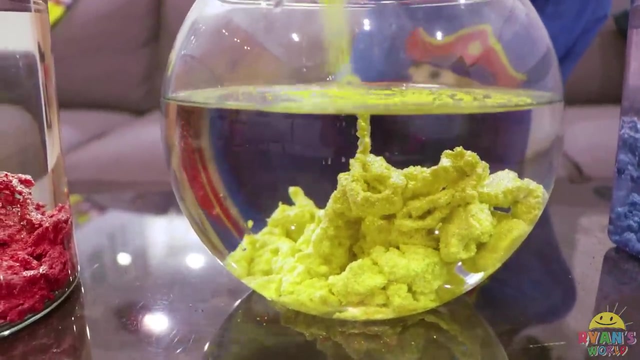 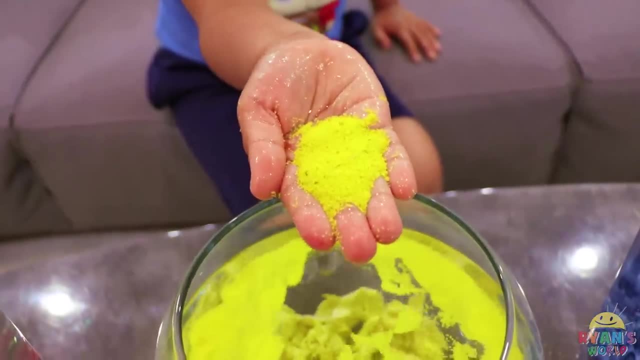 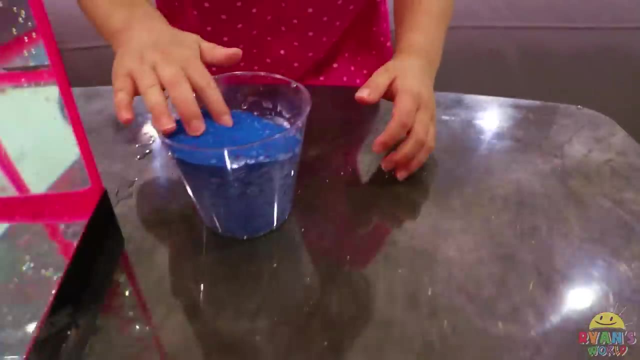 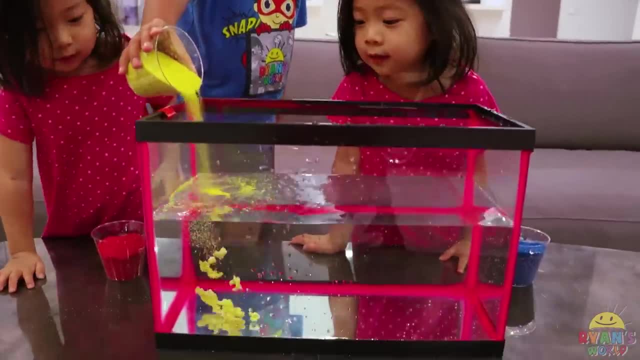 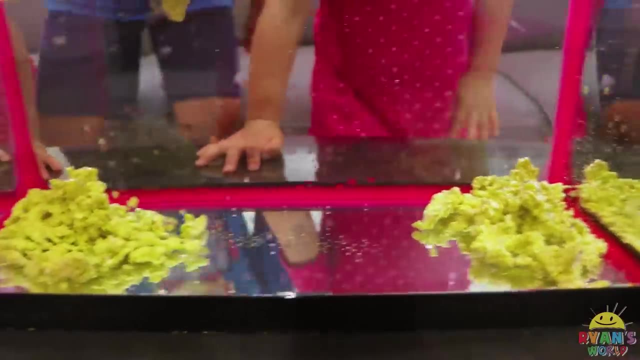 Okay, That's so cool. Slow, slow, slow. Let's watch it. Whoa, Look how it comes out. it looks really cool coming out. Whoa, Mom, can I do it now? Yeah, who's next Me? 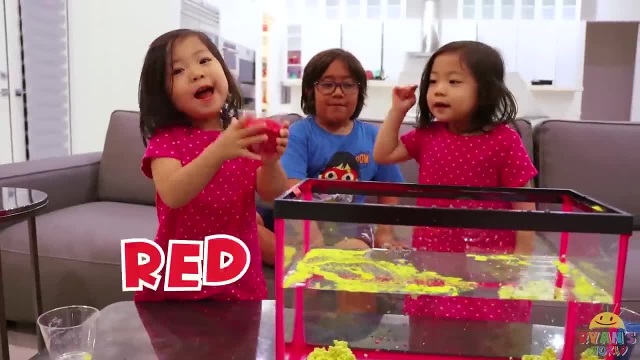 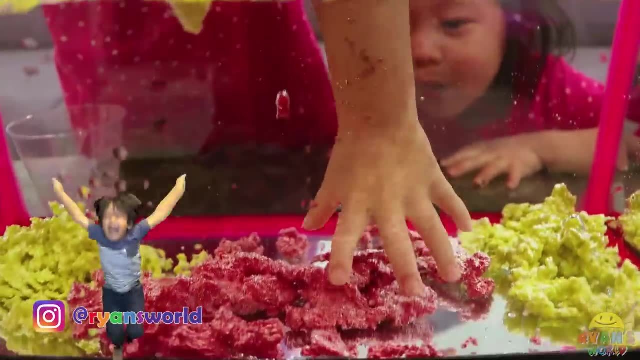 I'm already ruling the ocean Me. What color are you doing, Kayla? Yeah, Red, Uh-huh Blue. Yeah, put it in there. Whoa, keep doing it fast. Whoa, Yeah, I don't want to put my hand in there. 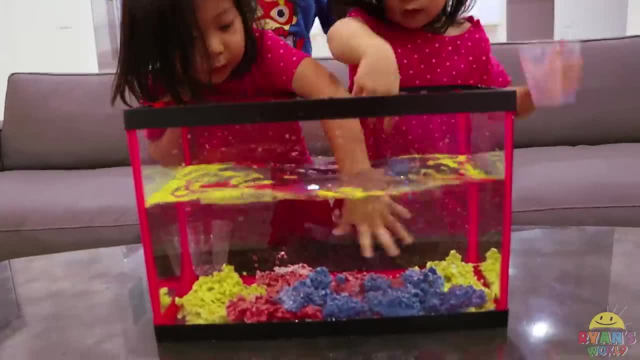 No, it's my turn. Yeah, Emma turned to do blue Whoa, Whoa. okay, so Emma, put it in there, Mix it together. You didn't get to record in time, Okay, So I'm gonna mix it. 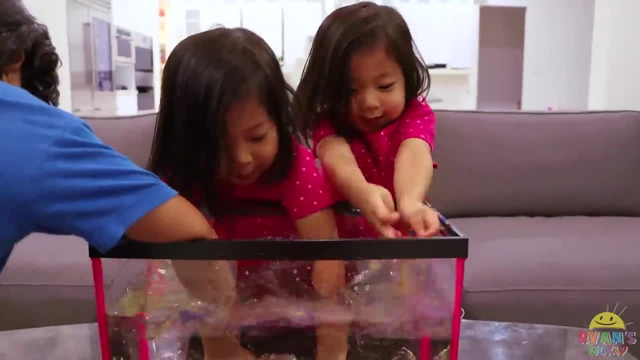 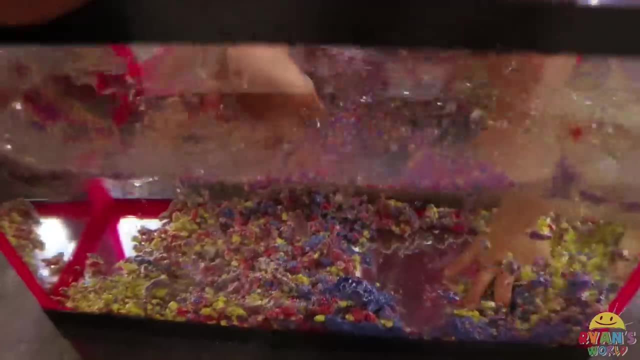 That's what it looks like together. Yep, It's rainbow. Yes, Is it rainbow? Yeah, it has winkles. Look at the winkles. It's rainbow. You like it? Yeah, When you pick it up, it's dry right. 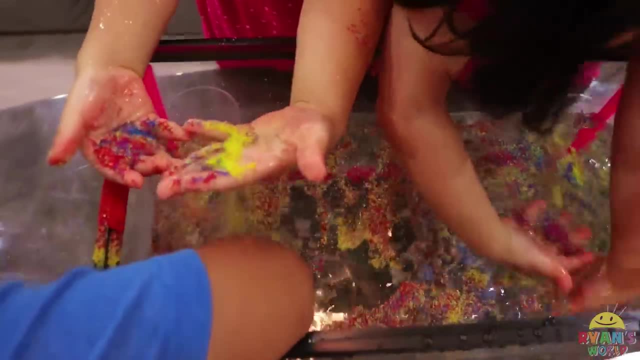 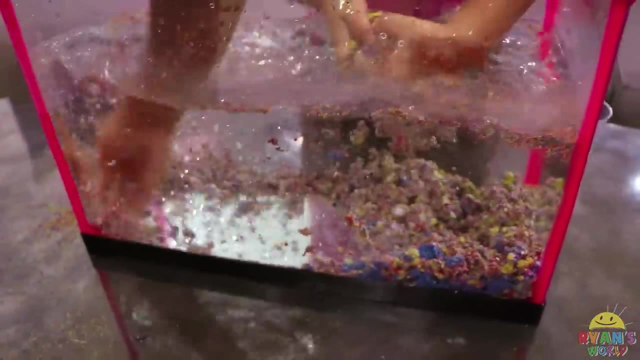 Yeah, All right, let's pick it up and see Whoa, Whoa, it's dry. when you pick it up, Tornado, Tornado, Ryan, I'm gonna pick it up for you guys to see Whoa. 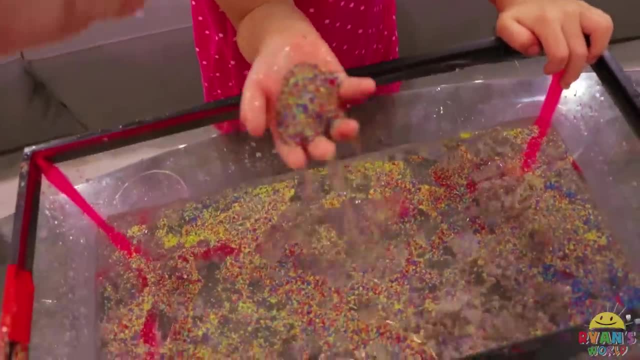 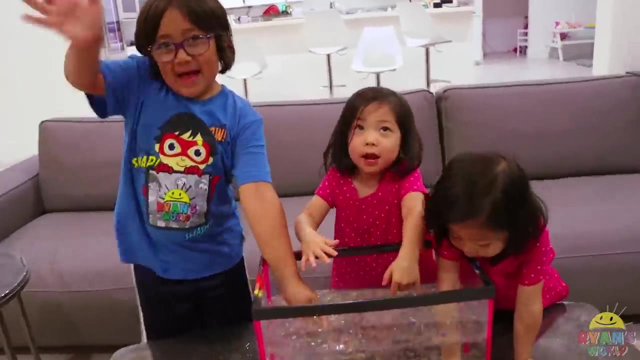 Mommy, don't pick on me. She, she, she, she. There it is Kate, Cool, huh, Yeah, it's very cool. Bye, Bye, Bye, guys, Hope you liked our science experiment. Bye.